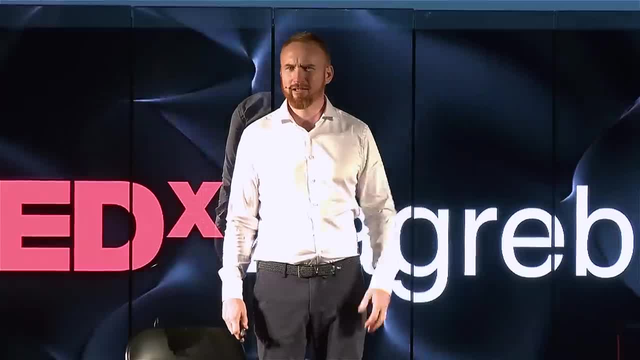 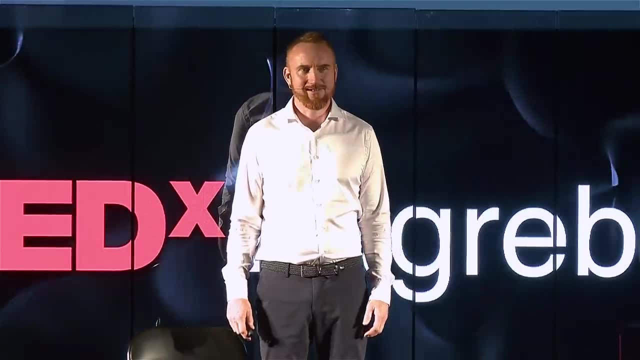 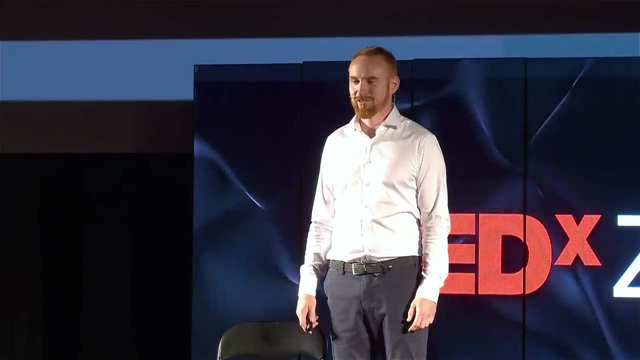 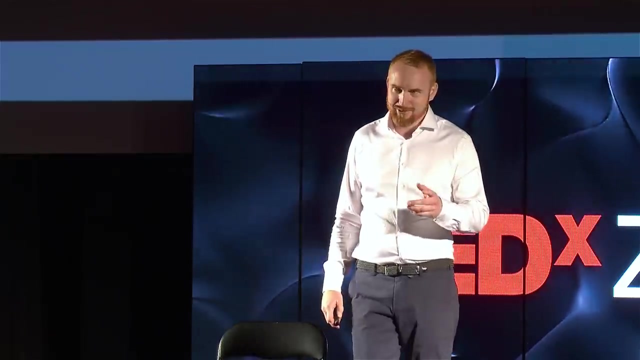 and understand what makes a good speaker good, what makes a great speaker great and what makes an outstanding speaker outstanding. The result: 110 core skills with loads of sub-skills. So what does it look like? It looks like this: 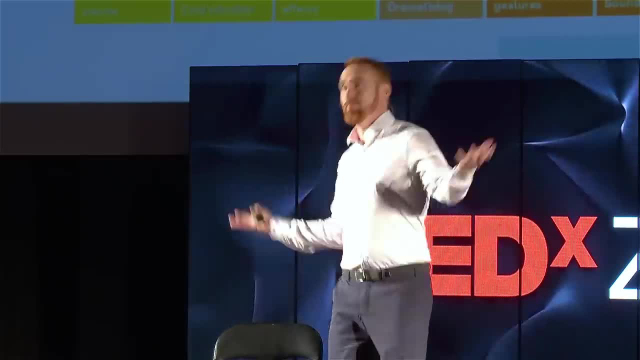 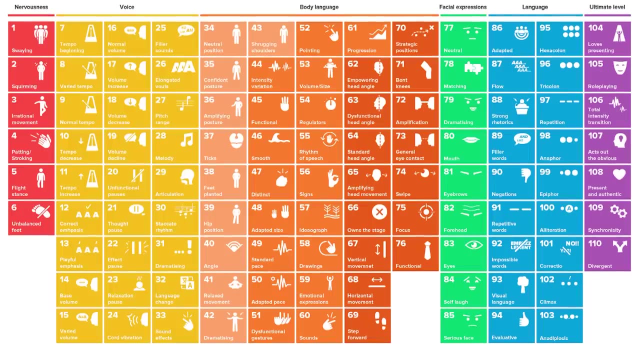 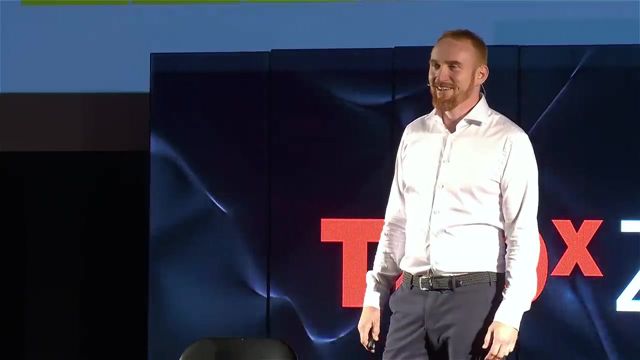 110 core skills, and the equation is simple: The more of them you fulfill, the greater you are. Now, 110 skills- that's quite a tad too many to go through in one TED talk, don't you agree? So what I've done is I've picked out my absolute favorites, and I'd like to 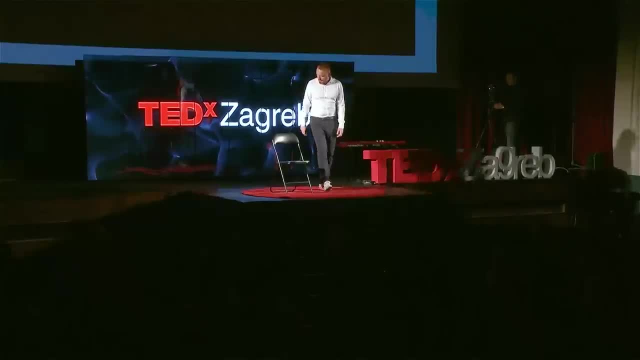 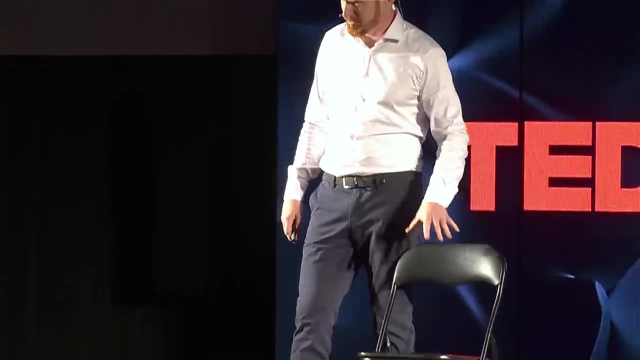 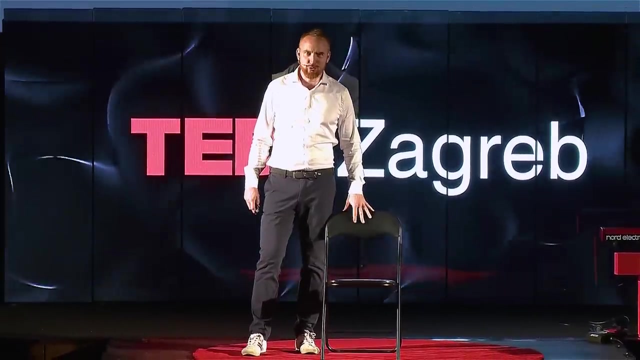 show you a demonstration of what it can look like, So you can see that the chair is something that you want somebody else to believe in. You want somebody else to buy into this. This is your idea. This is you wanting to make your voice heard. This gives you two options: Either you're on this side of the 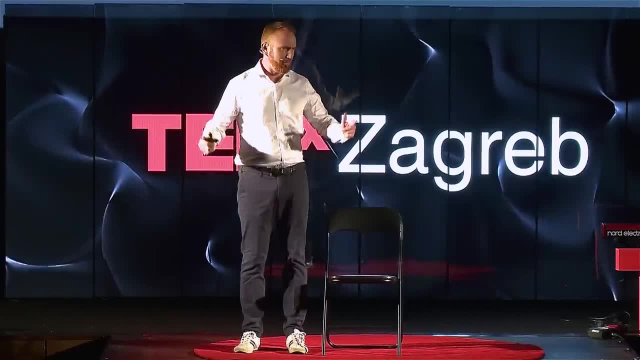 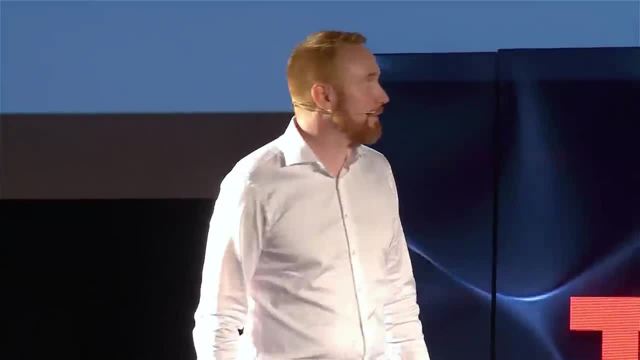 chair and you're a fairly mediocre communicator. you shoot from the hip, you hope for the best and sometimes it works. sometimes it doesn't. Option number two is that you're on this side of the chair and you know exactly what you're. 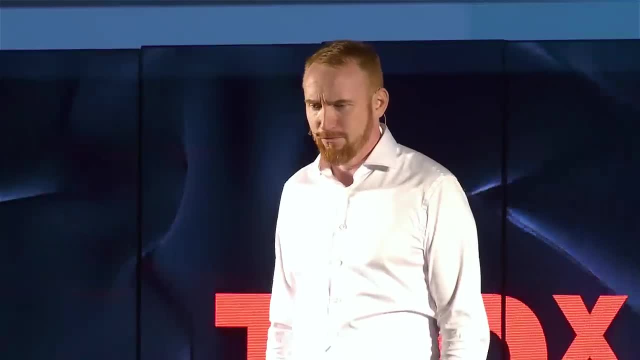 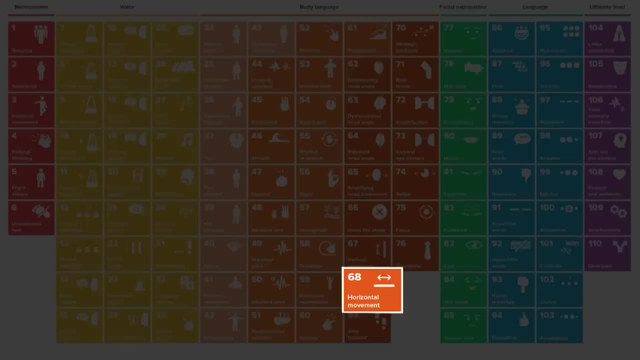 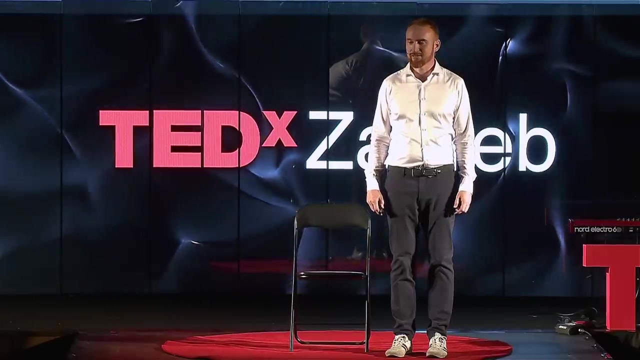 doing in every instance of time. You know that by taking a step forward, you increase focus. You know that by tilting your head slightly to the side, you increase empathy. You know that by changing the pace of what you are saying, you increase focus And you. 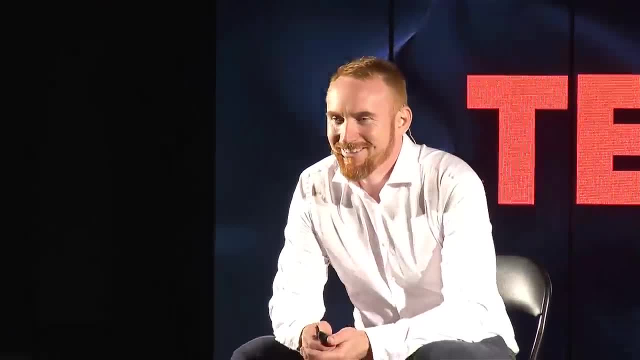 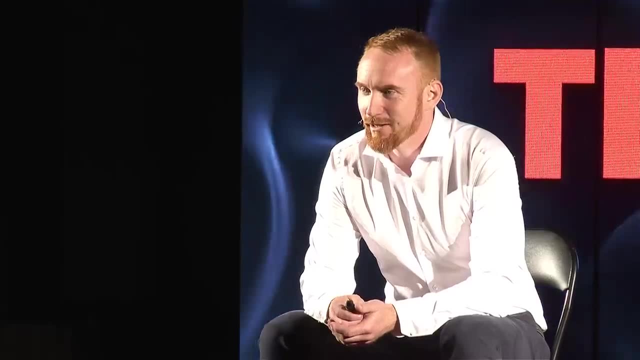 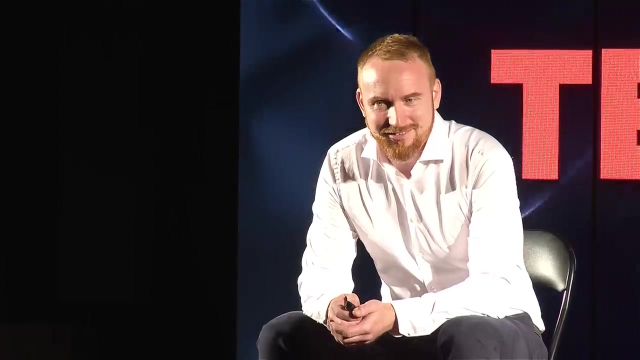 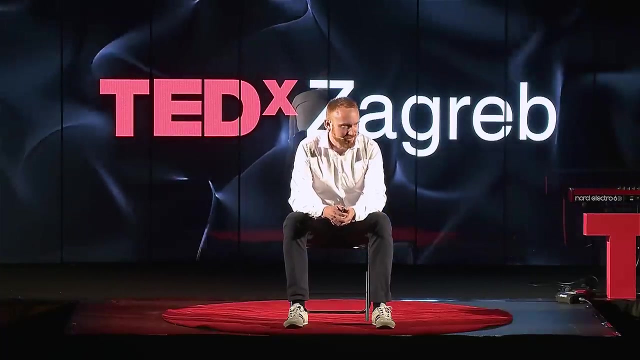 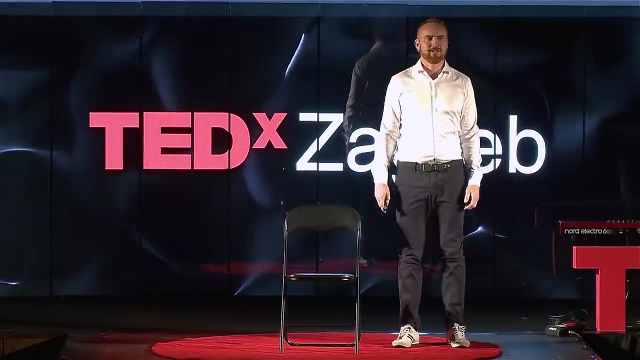 know that by shifting yourself lower, you increase trust. And you know that by lowering your voice you increase confidence, You get anticipation. And you know for absolute certain that if you pause, you get absolute and undivided attention. Now the question then is: can everyone be on this side of the chair? Can everyone become? 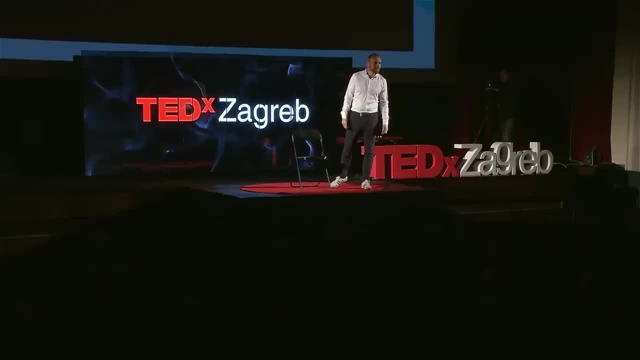 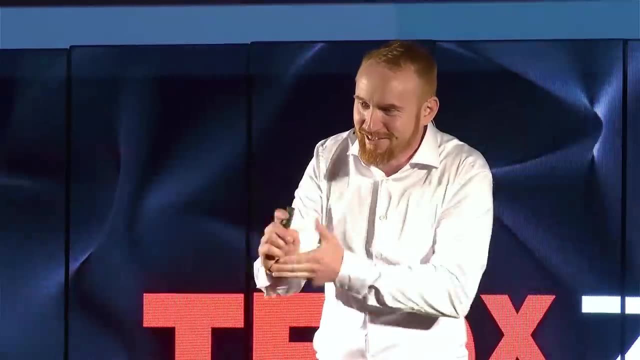 good at these skills? What do you think? the answer is, Of course it is Why? Because it's called presentation skills, skills, skills, skills, skills, skills skills. It is not, has never been and shall never be called a talent. You're not born with a particular 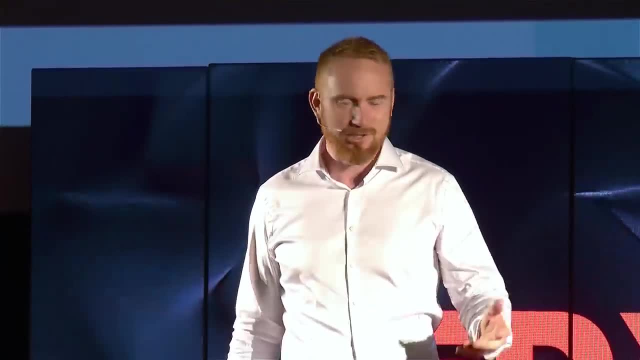 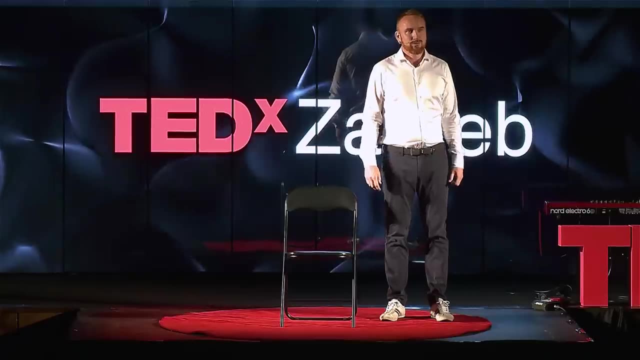 gene that makes you brilliant on stage. It's something you acquire through life. Now, as I said, 110 skills- that's quite the number. So what I've chosen to do is I've picked out the five, would I say, most important skills. Whenever somebody comes to me and 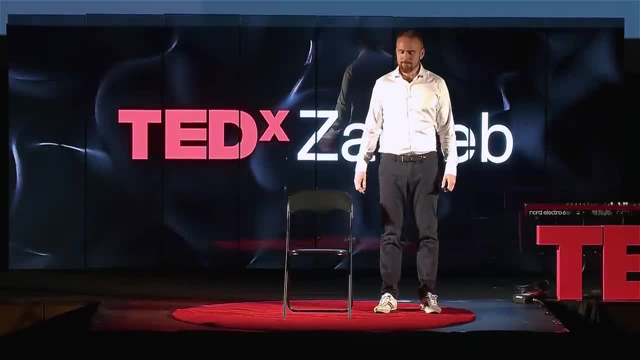 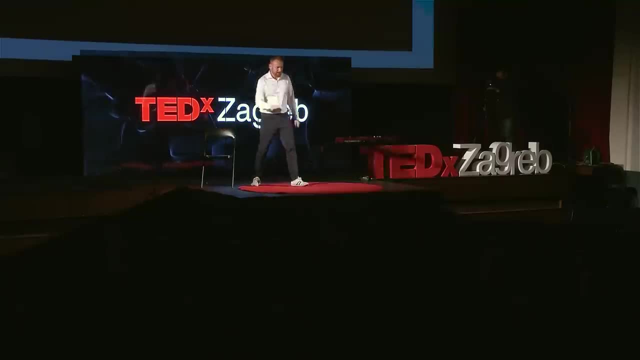 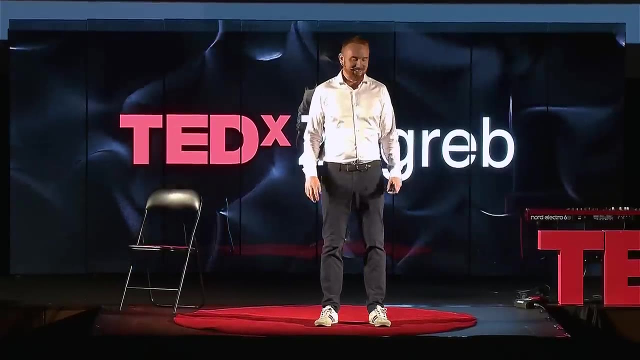 they want coaching. this is what I focus on, And then I'll actually give you four bonus skills at the end as well. Sounds okay, So let's start with two of my favourites from body language, which is skill 34 and skill 69.. That is not intentional. 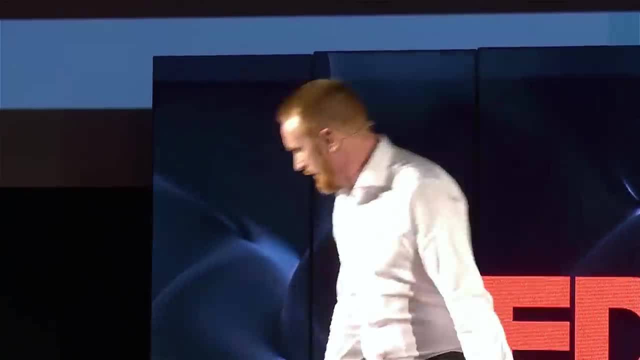 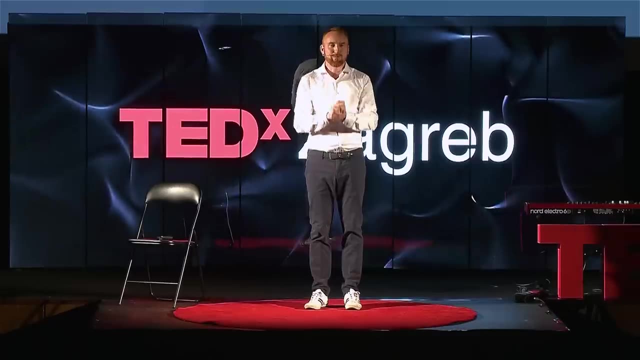 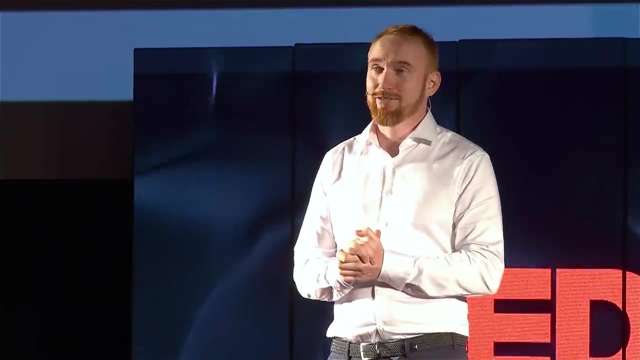 Now 34,. what am I doing? What could I be doing differently in this case? Ladies and gentlemen, it is an absolute pleasure to have you here today. Good of you to come. What should I have avoided? I should have avoided closing my body language because 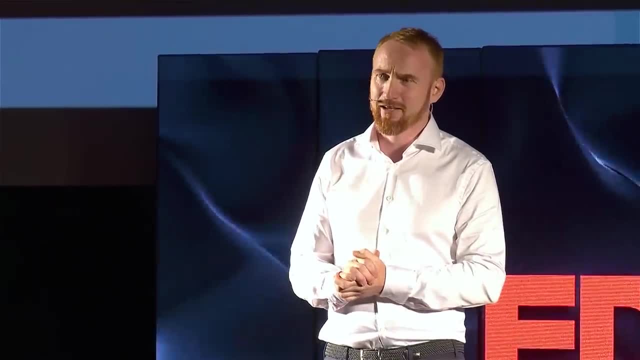 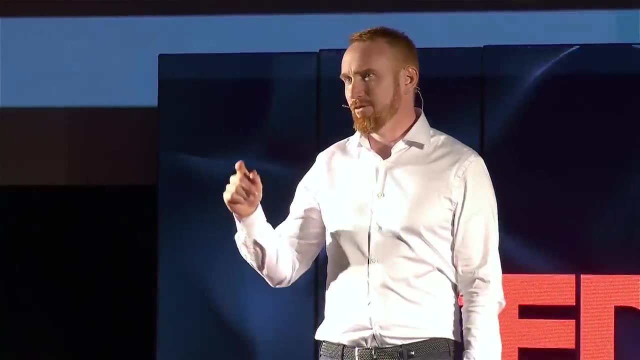 whenever a human being closes their body language, it is a sign that they feel threatened in one way or another. So I should have continued with an open body language. So let's have a look at number 69,, which looks like this. I'll have to start up here, So 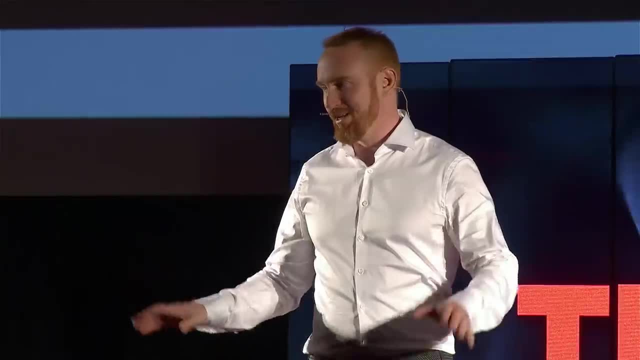 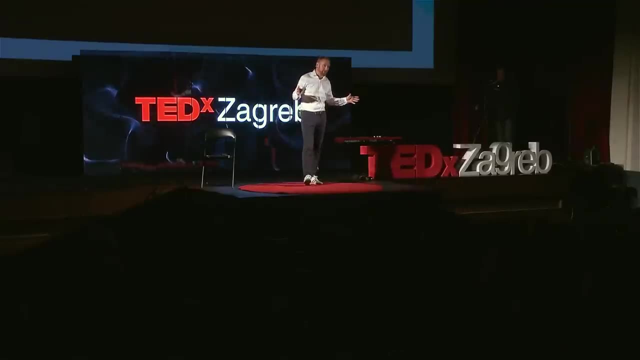 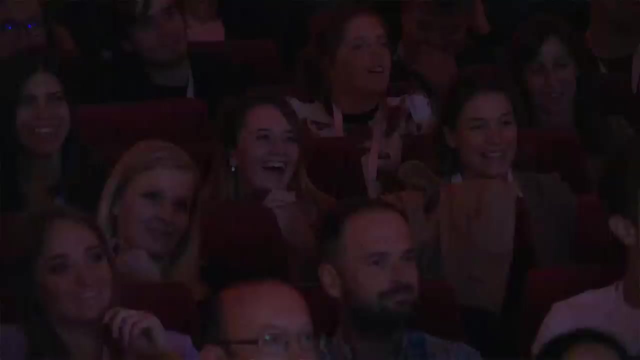 when a presenter starts like this, they go: what should I do better now? Ladies and gentlemen, welcome to one of the most influential subjects known to mankind. Now, this will be super interesting. We'll be going through this. You'll be having an amazing time. Wow, it'll blow you away. 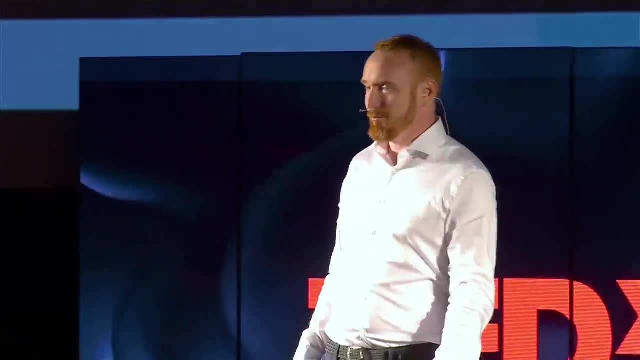 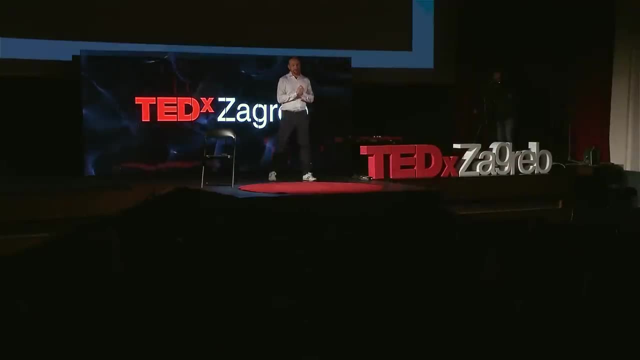 What should I have avoided Reversing? Look what a double incorrect looks like. It looks like this, Ladies and gentlemen, absolute pleasure to have you here. Good of you to come. Well, a double correct looks like this: Ladies and gentlemen, an absolute pleasure. 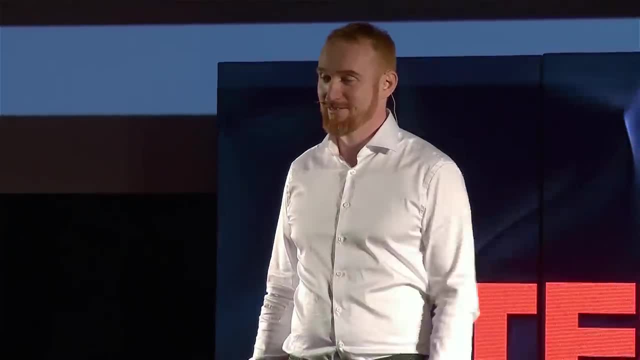 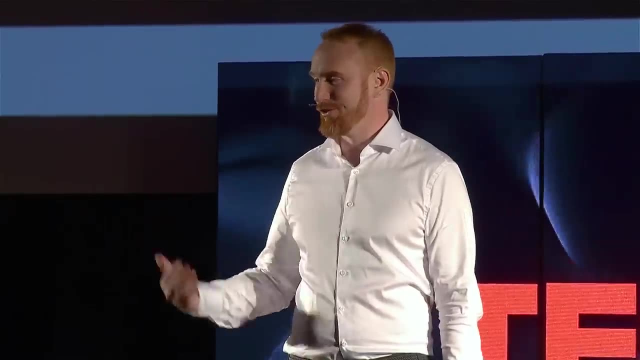 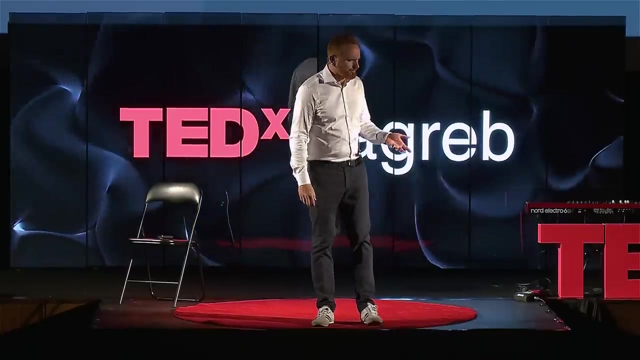 to have you here. Good of you to come. Is there a difference? Of course there is. The biggest difference Is in here. I can feel a difference. while doing those two versions, You become what you are. Now let's ask ourselves: yeah, but David, the closed body language thinks what? 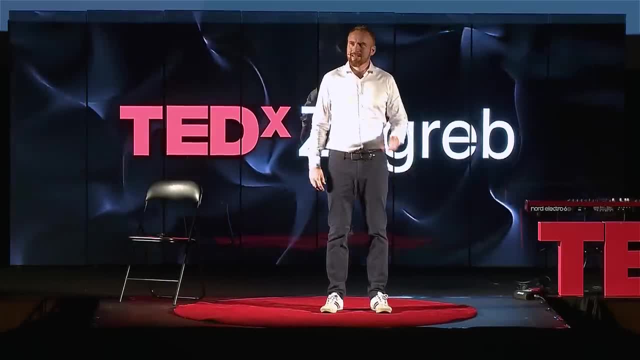 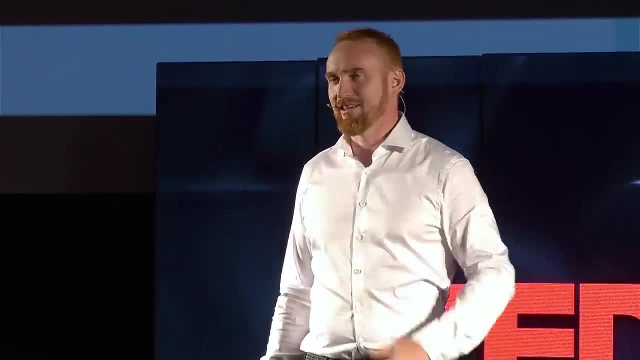 shall I do with my hands? Where shall I put them? And the interesting thing with the closed body language is that wherever I went all over the world studying these people, it seems like we've got a general kind of locked body language positions. 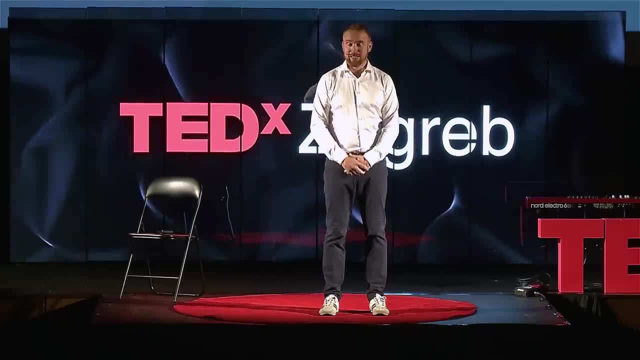 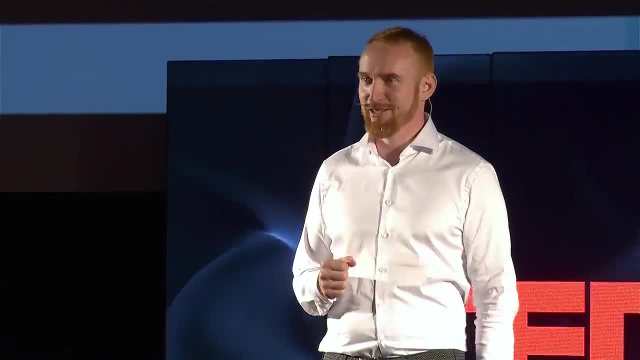 and I'll show you my favourites that I've found. We've obviously got the classical fig leaf position. Then we have the double bunny position. You have the right bunny position, the left bunny position, the right huckle, the left tackle. 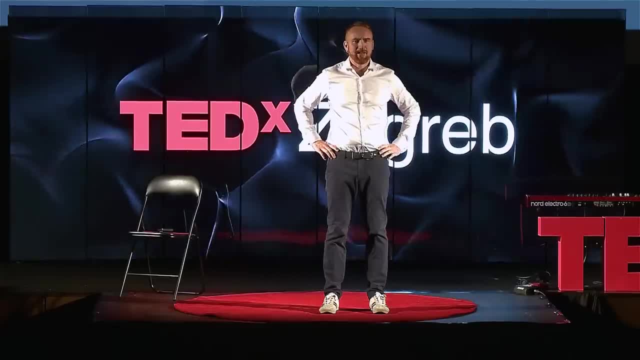 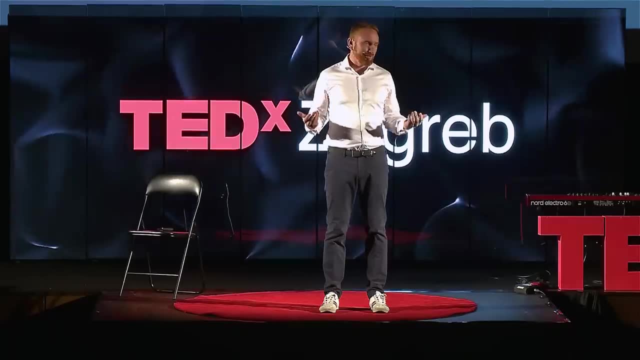 Then you have the forklift. You of course have the peacock with flapping elbows, You have the major, the merkle, the prayer and the beggar. One of my personal favourites is the British horse rider And the British horse rider. 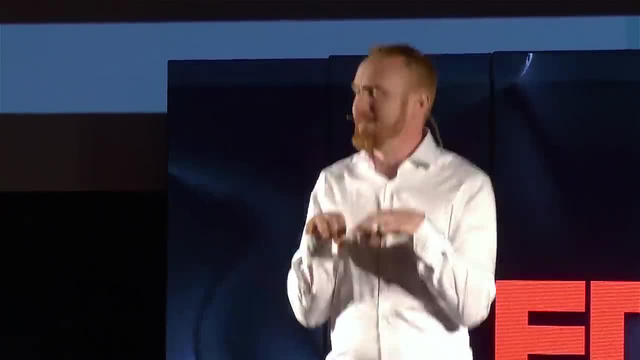 it's a person who holds their hands like this, puts it just above their chest and it's like they're off somewhere. Oh God, there are foxes over here. And then we found two T-Rexes as well in the study. 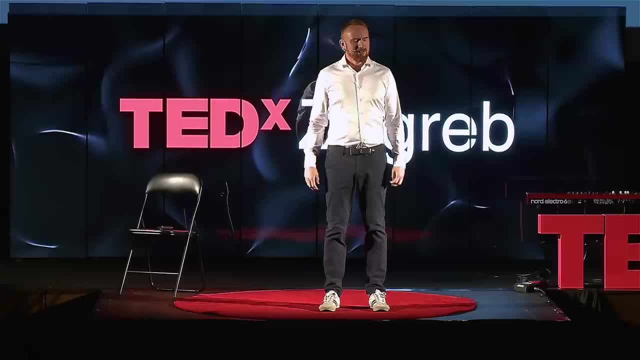 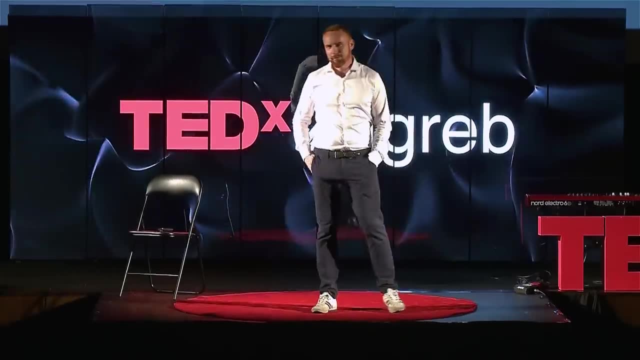 Such a weird thing, presenting like this or like this: Okay, so you mean, David, that we need to have an open body language? Yeah, that's what I mean, And I'm not allowed to have them in my pockets. 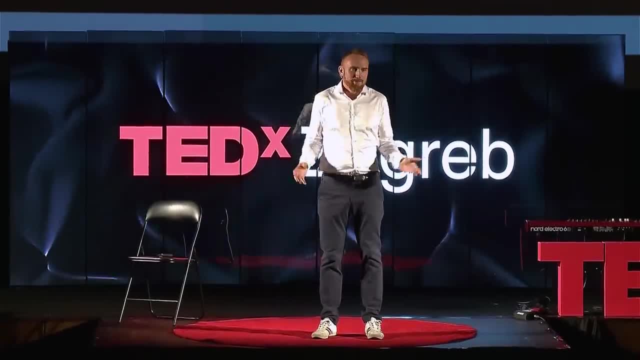 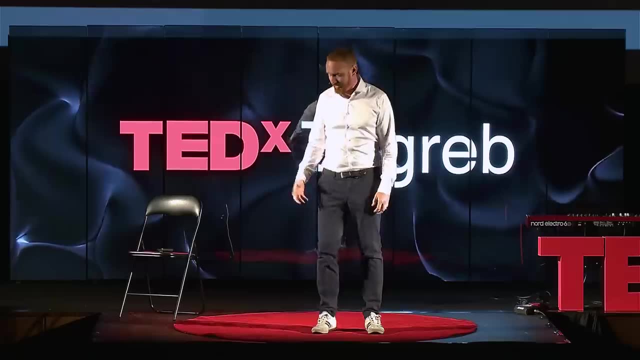 not allowed to have them in my major or the double bunny? No, But what on earth shall I do with them then? What you should use them for is what is called fungiboying- Functional gesturing, to show that something is getting better. 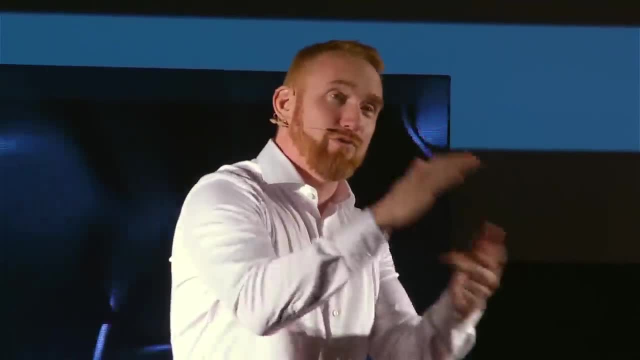 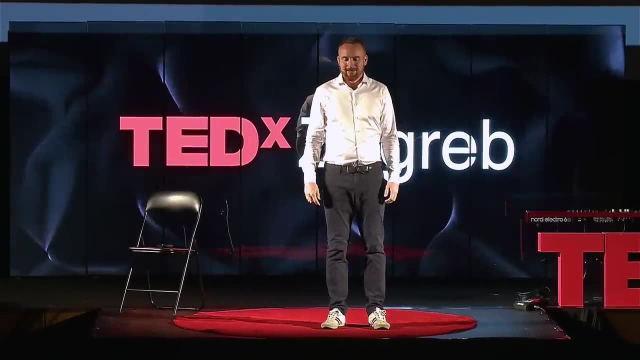 or that something is getting less good, or that it's one, two, three, four, five that we are going to go through. Use your gestures for what they're supposed to be used for, And what's interesting with this is that, if you imagine the time we've spent on this planet, 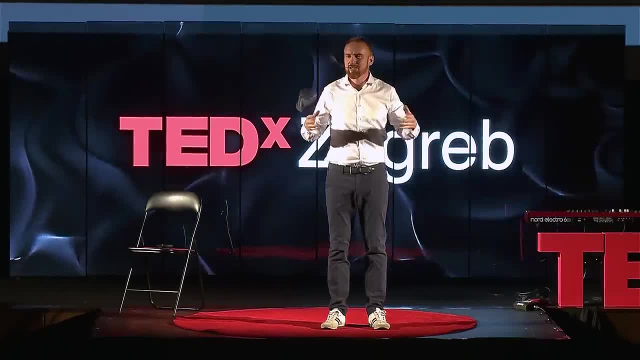 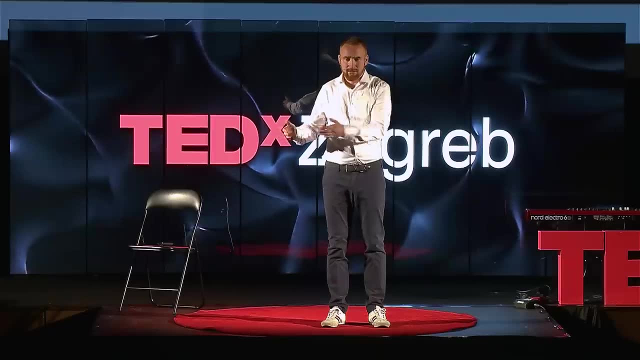 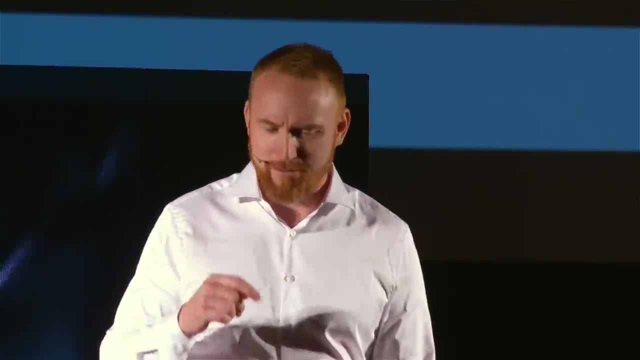 as our race. how much of that time have we spent using gestures and non-verbal communication in order to communicate what we're saying? Is that more than verbal? Absolutely, So. let me give you a demonstration of how important it is. So I'll say something now. 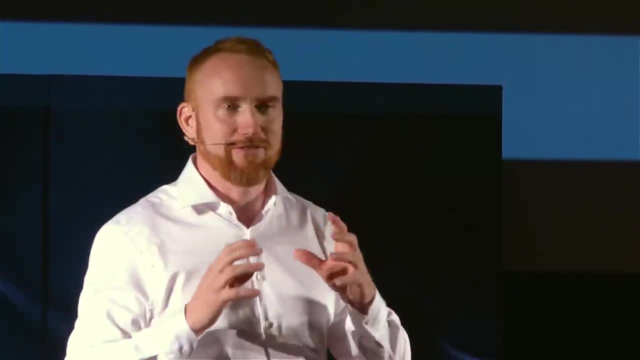 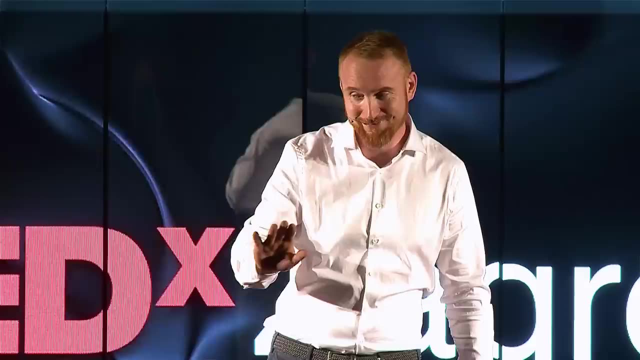 and everything I say will be super positive. My facial expressions will be super positive and the way I say it will be super positive, but my hands will be saying the opposite. Are you with me, Because this requires some focus? All of you should learn more about public speaking. 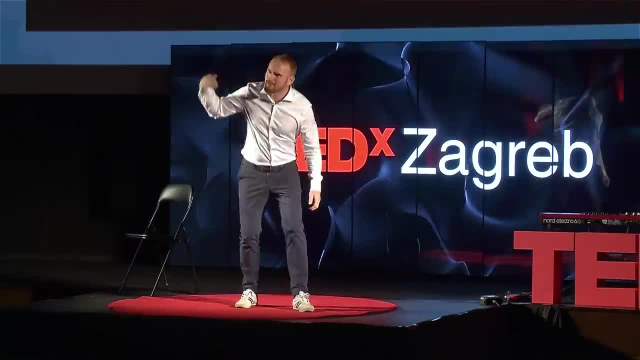 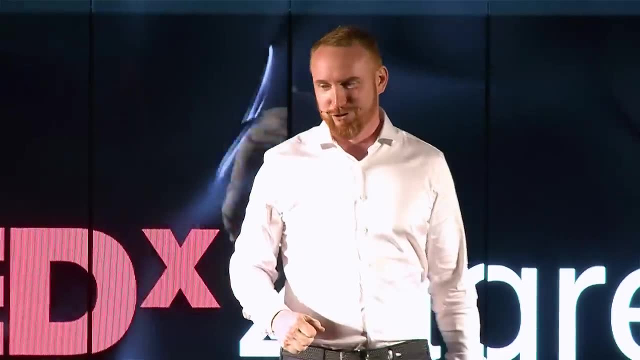 because if you do that, you will become better, You will grow and you will develop as a human being. People will love your presentations, listening to your arguments and just generally loving whatever you're doing. So do yourself a great favor. 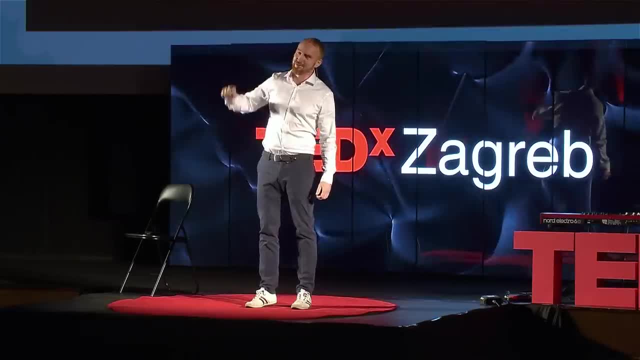 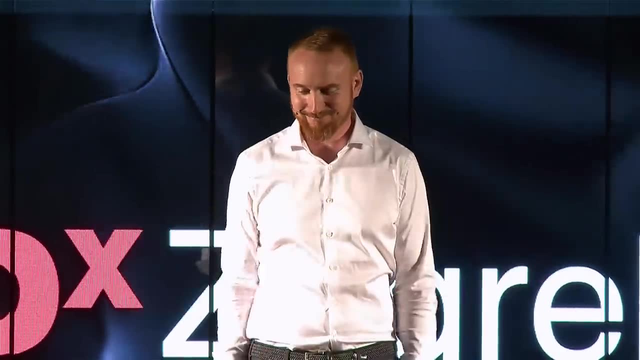 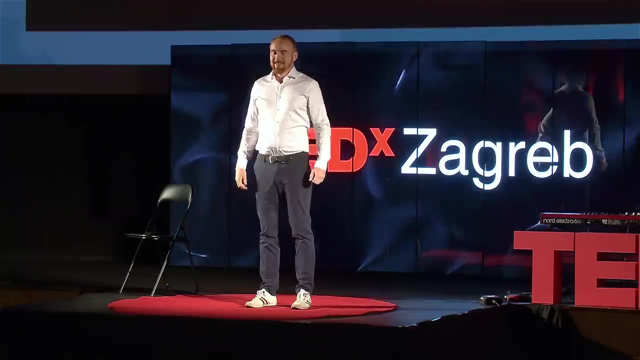 Learn more about this particular subject, because you'll be thanking yourself for the rest of your life, And particularly you have been absolutely incredible, so I thank you for listening here. Now the question is this: Did you listen to what I was saying or what I was doing? 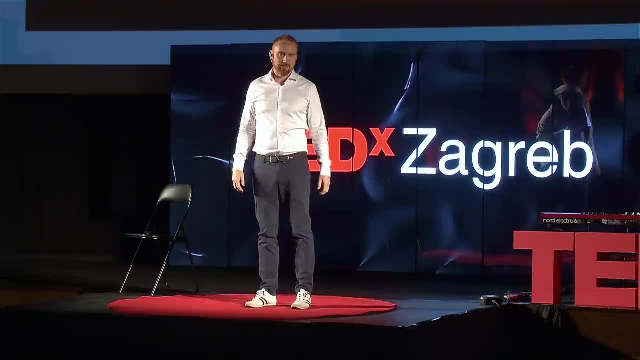 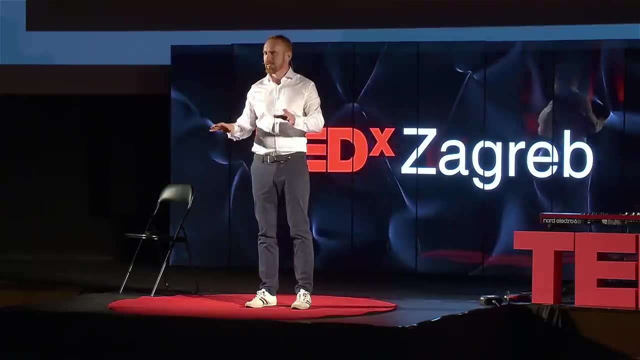 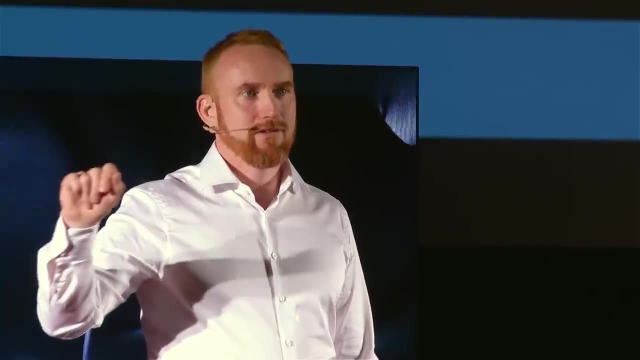 I believe that you focused entirely on what I was doing, and that is the case with body language and gestures. If it's not saying the same thing as what you're saying verbally, there's a discrepancy and a disturbance in the communication. Let's move on from body language to a couple of tips on voice. 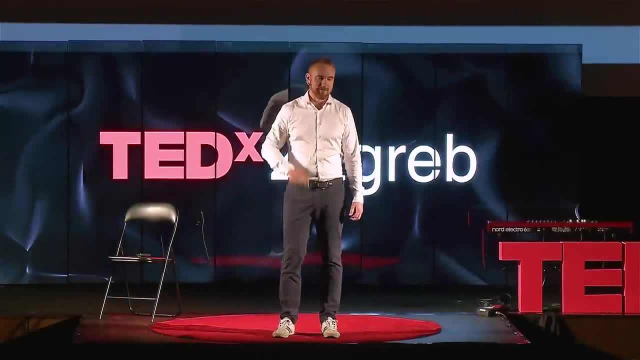 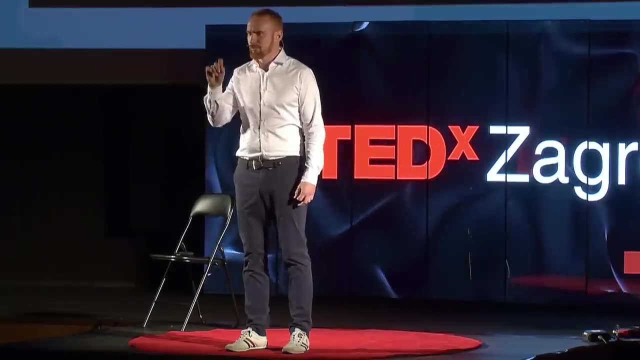 And the first one I'm going to give you is about pace. So listen to this, Ladies and gentlemen: what I'm going to take you through now is incredibly important, now and for the rest of your future life. We'll go through the cortex, we'll go through the limbic and the reptilian system. 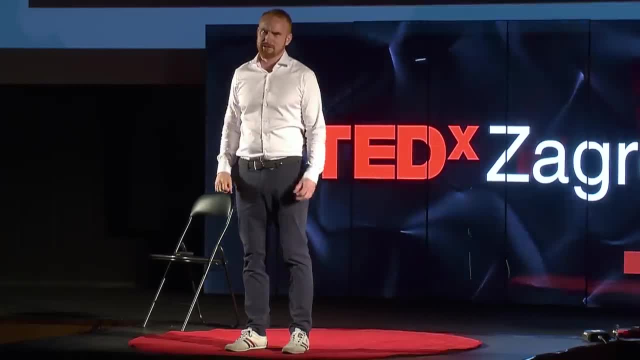 We'll go through a psychologically advanced profile where we'll take you through the entire steps of the structure. We'll then look at how that relates to Aristotle and see if there's logos and pathos, and I'll carry on in this pace. 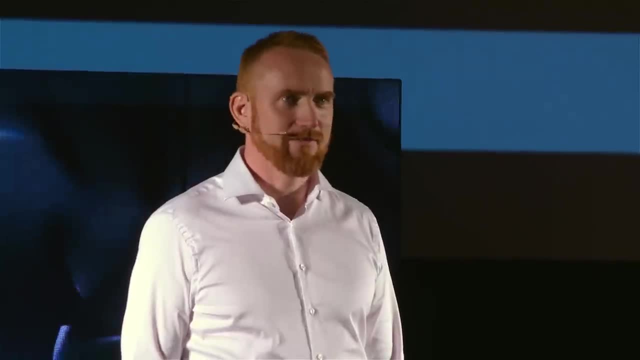 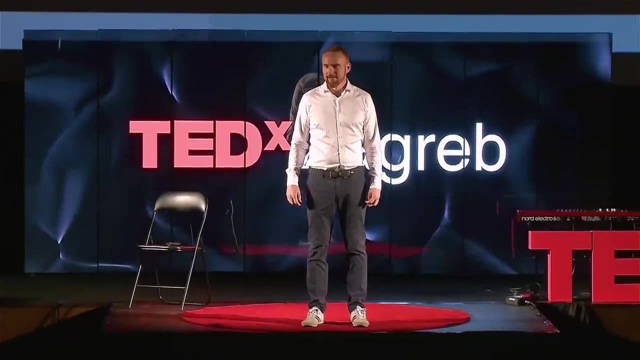 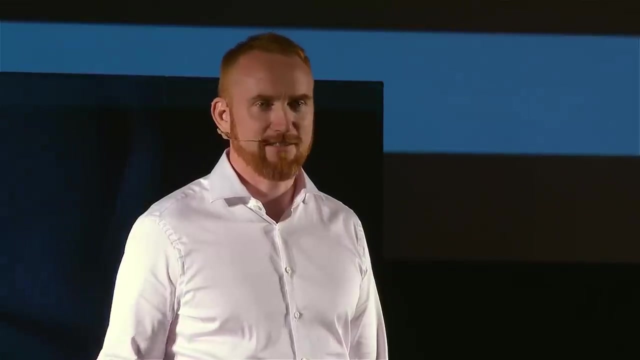 Compare that to this. Ladies and gentlemen, I'm now going to take you through something that is entirely and utterly boring, Something that you will have no use of in your entire life, And every second spent listening to me now and on will be a waste of time. 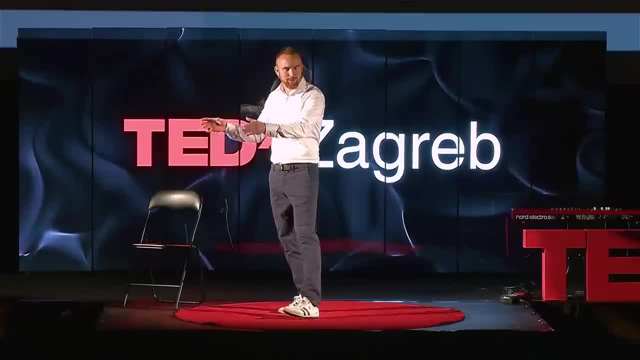 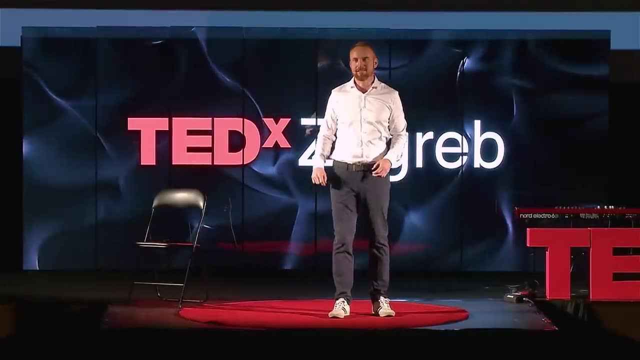 And now look at your faces. You're like, whoa, that last bit. I want more of that. That was super interesting. The useless stuff. I don't want the brain so much, I want the second bit. Why? Because your brains. they react to when a person has a low pace. 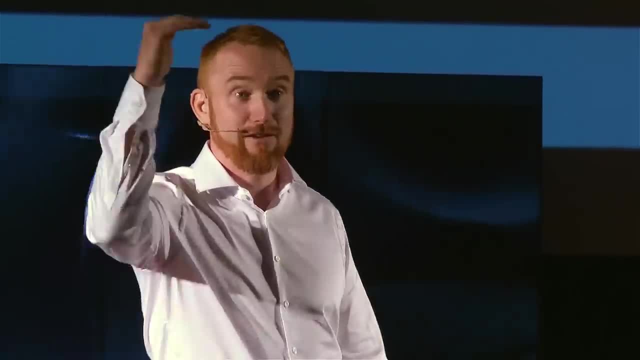 You think that what I'm saying is more important than when I have a heart attack? You think that what I'm saying is more important than when I have a heart attack? You think that what I'm saying is more important than when I have a heart attack? 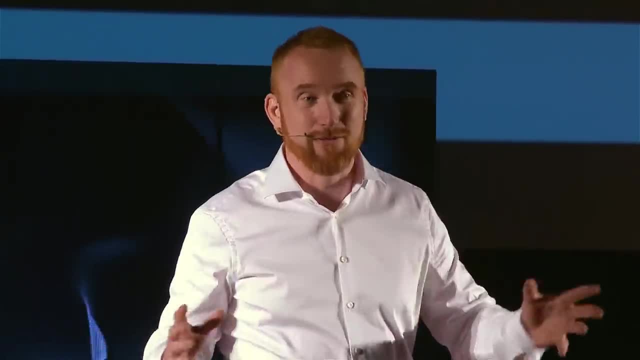 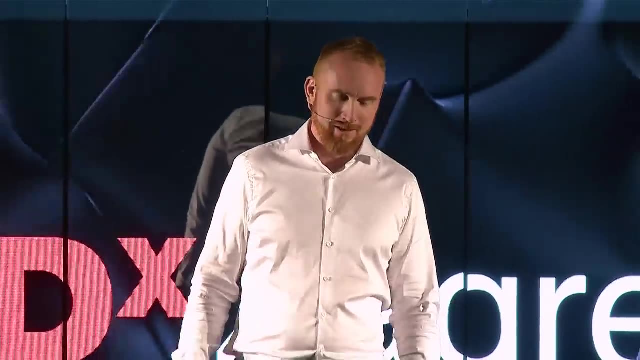 I'm not talking about a high pace, because that illustrates that I don't really want to be there. There are exceptions to this rule, but that is the basics, So keep a calm pace. My next tip goes on pauses: The pause. 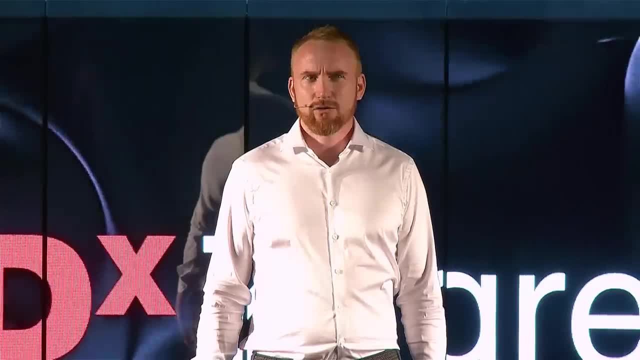 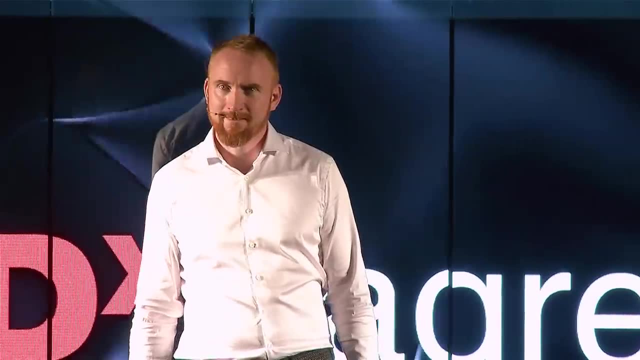 Is the pause important? Absolutely it is. So let me give you a classical rhetorical proverb, Now without pauses, And it goes like this: Did you know that every single decision you've taken in your entire life and will take for the rest of your life, 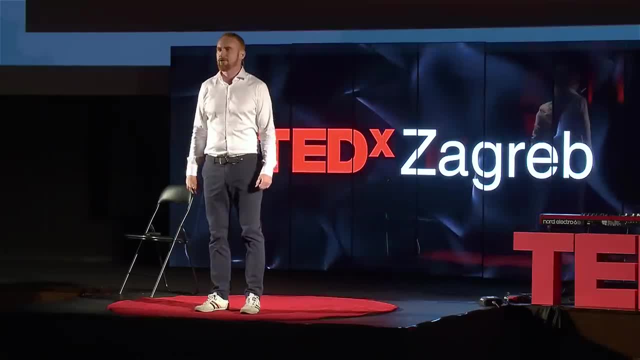 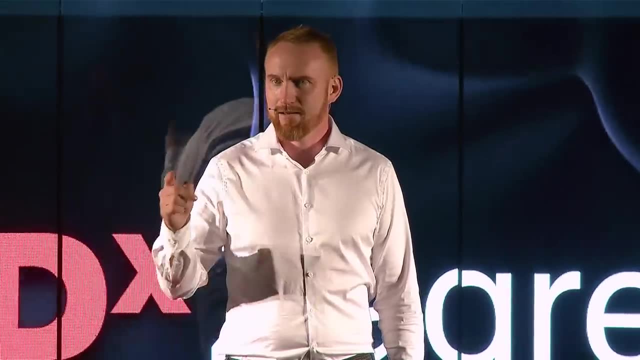 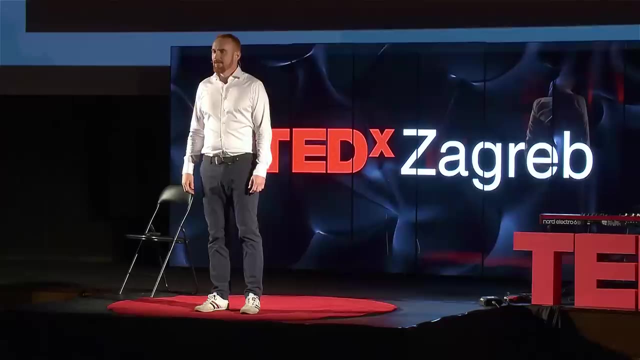 is based on one thing, and one thing only. If you give that to the people listening to you, that is the feeling, That is what will move them. Now I'll add pauses, And it sounds like this: Did you know that every single decision you've taken, 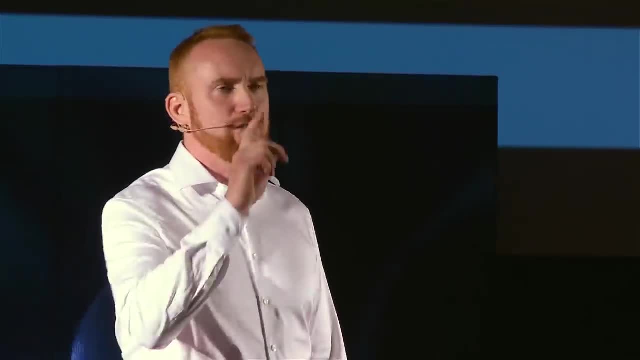 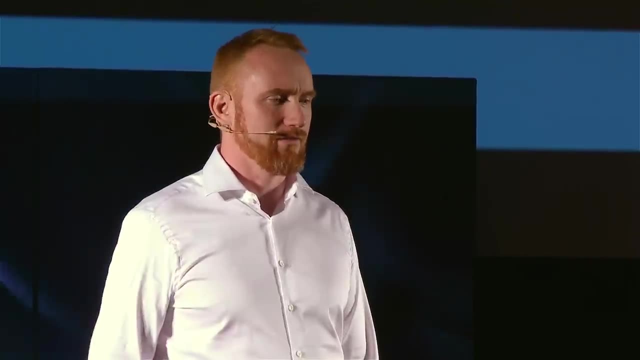 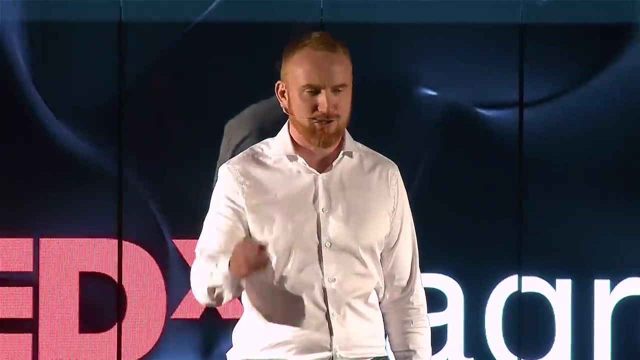 in your entire life, and you will take for the rest of your life, is based on one thing and one thing only, And that is an emotion. Now, if you give that emotion to the people listening to you, they will take the decisions you want them to take. 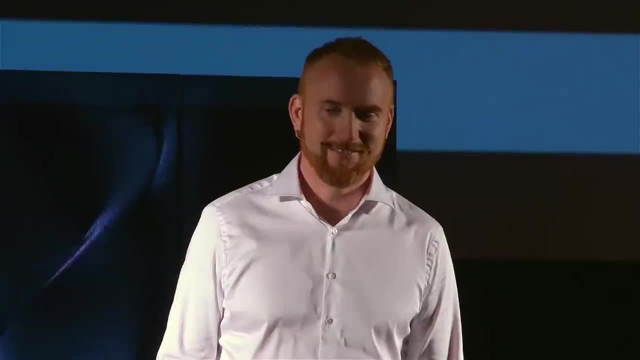 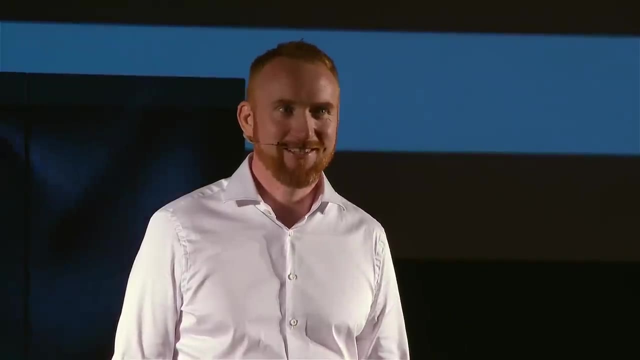 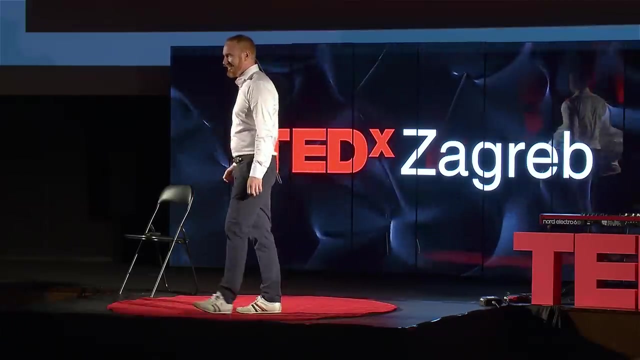 Is there a difference? Absolutely, But you know what. Some people are afraid of the pause, So they go like, whoa, Am I going to do one of those? I'm not. I refuse. I prefer to compromise. And do you know what the compromise for a pause is? 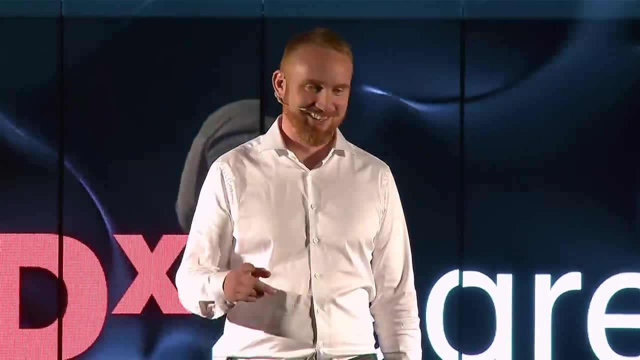 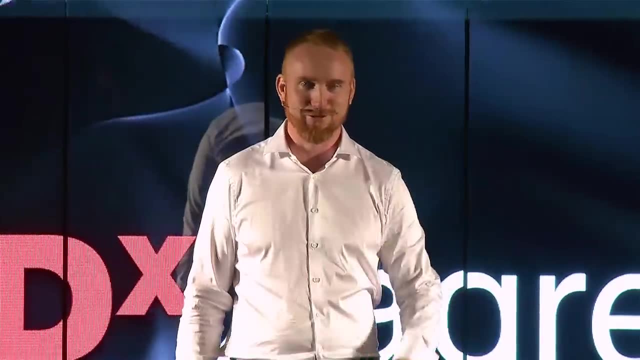 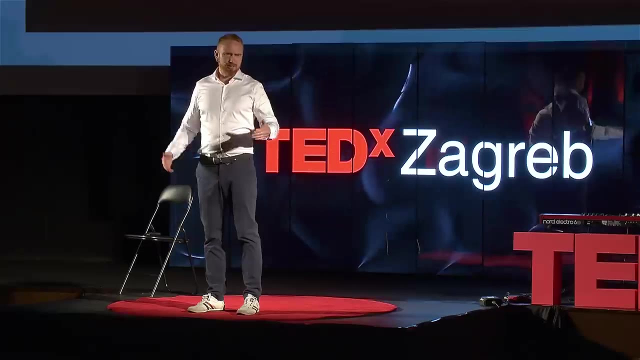 What does it sound like? Uh yeah, Uh eh, Ah bleh, It's like a skok of sheep when you listen to certain conferences. Eh, eh, eh eh. Now there's nothing among these 110 skills. 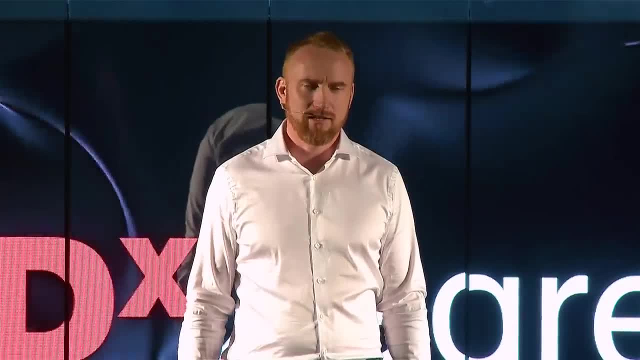 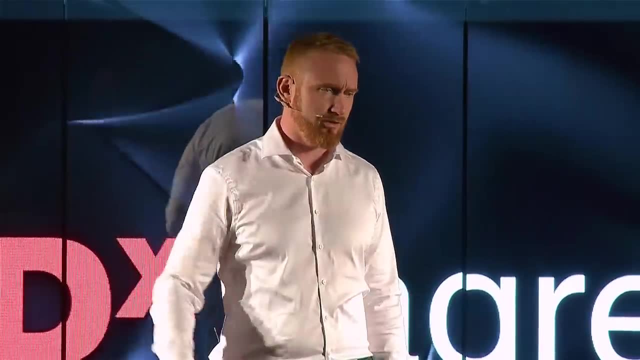 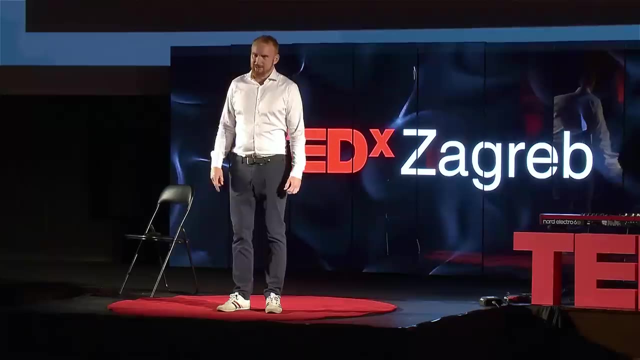 that lowers your ethos and your credibility more than uh uh-ing, Because it signals that you don't know what you are saying and where you're going in your talk. So let me give you a demonstration. Did you know that every single decision? 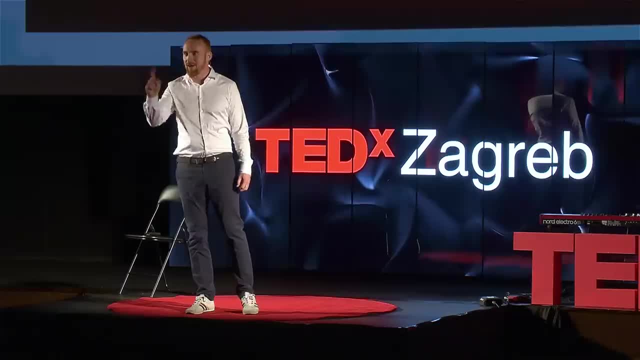 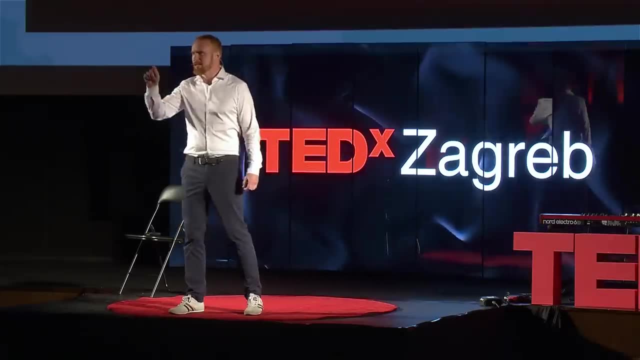 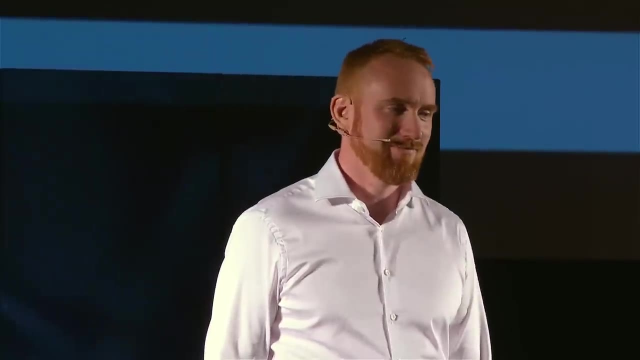 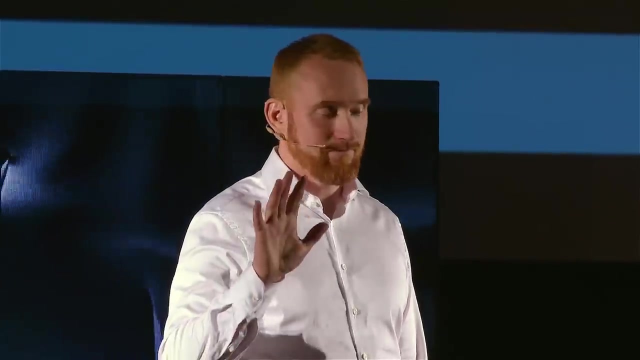 you've taken in your entire life and will take for the rest of your life is based on one thing, and one thing only: Uh, Uh, And that is a feeling. Uh, I think you prefer the one with silence. Now, those were the five main skills. 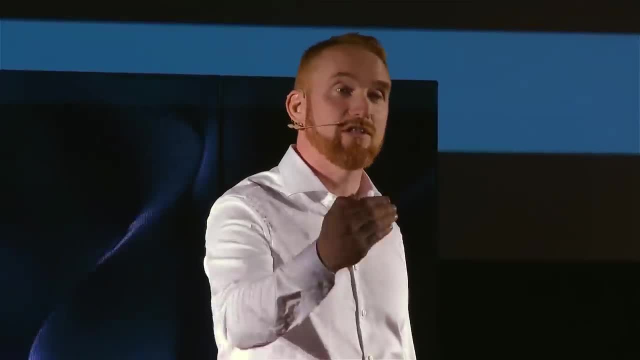 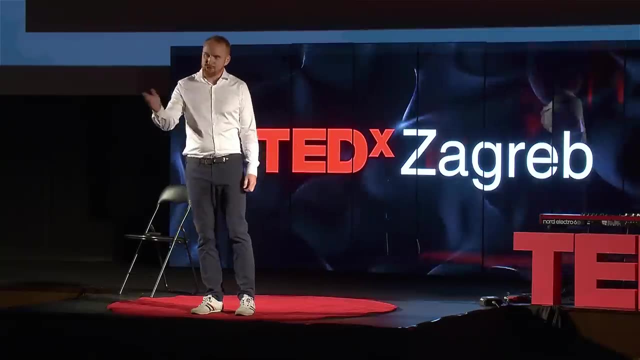 I wanted to take you through, And if you haven't used them before and you start using them as a public speaker, they will make a difference to your speech. I would like to treat you to four small skills as well, just to give you an appreciation. 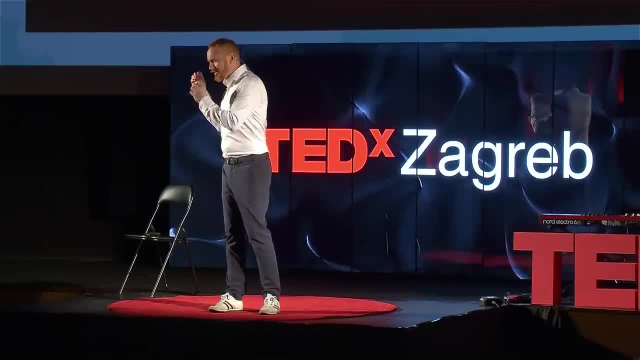 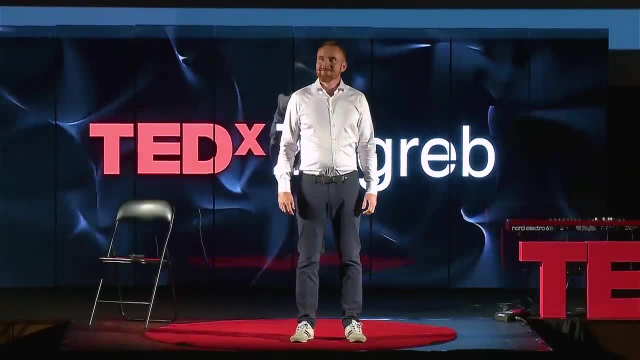 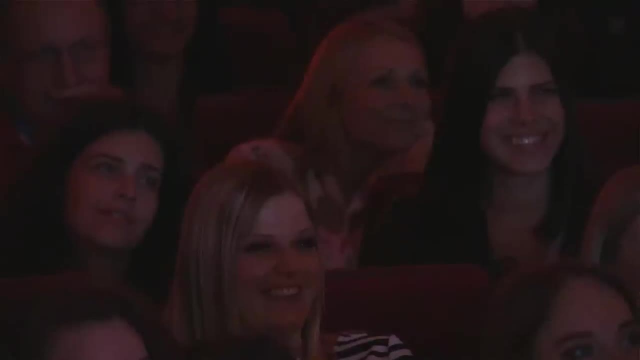 of how small a skill is. Small a skill can be, but still have a great impact. And it looks like this. And those were the four skills. Did you follow them? Number one, as I looked up, which illustrates that I'm thinking, 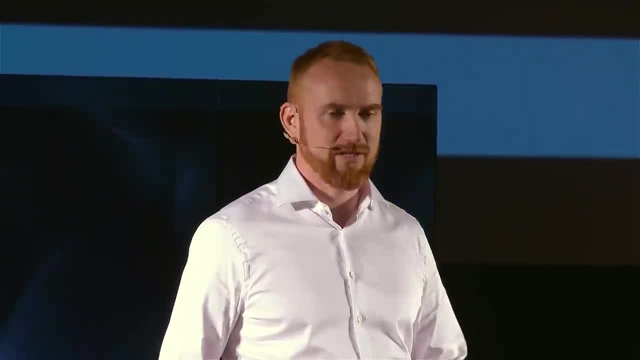 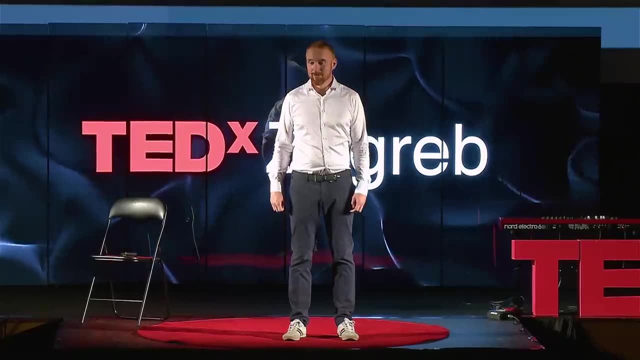 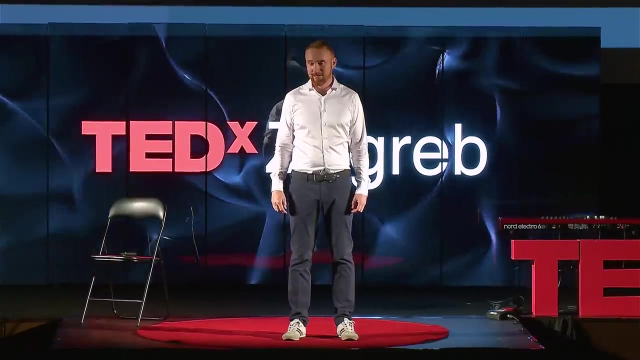 which increases your, your sense of presence for me on stage. The second thing I did was that that I did a audible inhale which makes your brain believe that I'm going to say something that's exciting. I then combined that with a Duquesne smile. 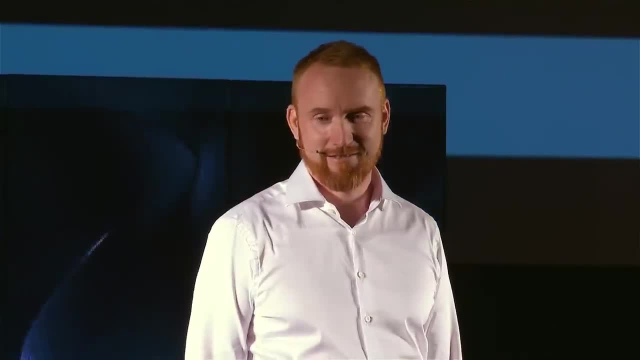 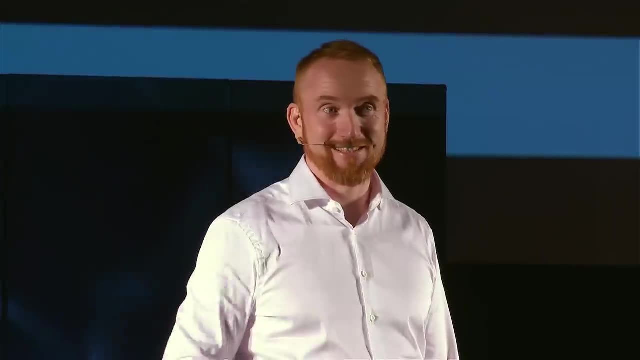 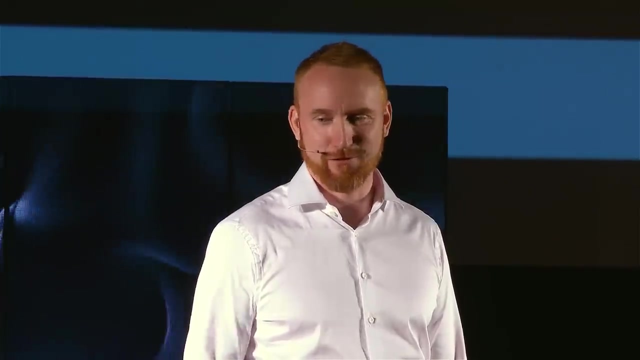 which means that I smile with my mouth and with my eyes. Did you fall for it? Because what I did as well was this: I did a self-laughter, And also that increases anticipation of what I'm going to say. So four small skills executed in five seconds. 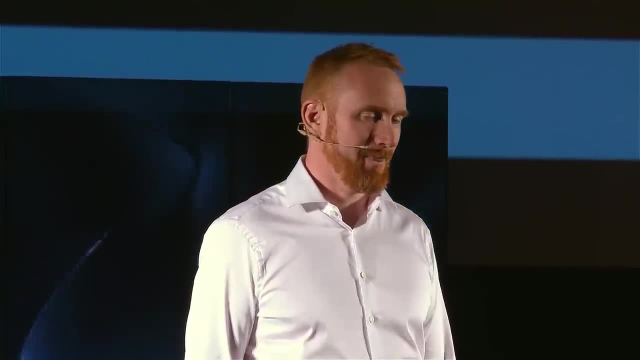 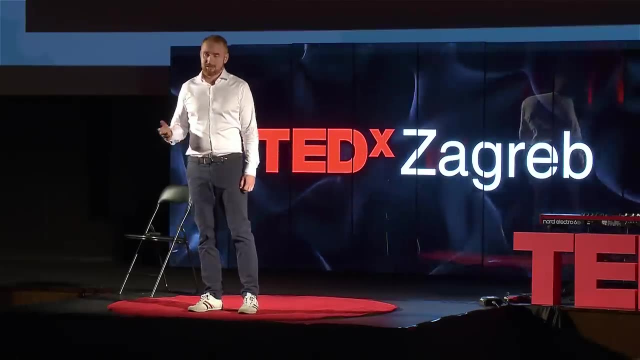 changes the state of your mind. I'd like to pick out one of those and just end off with that, And that is the Duquesne smile. Duquesne smiles has, in studies, shown that you are more likely to be married, less likely to be divorced. 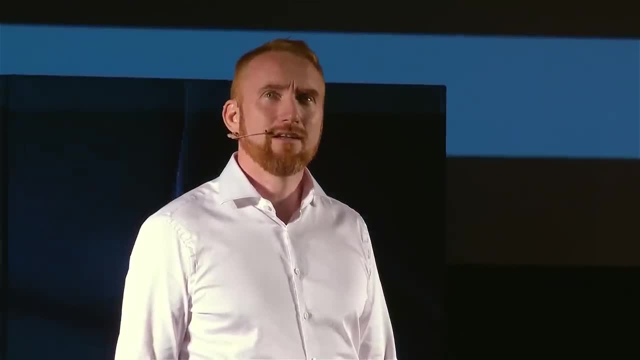 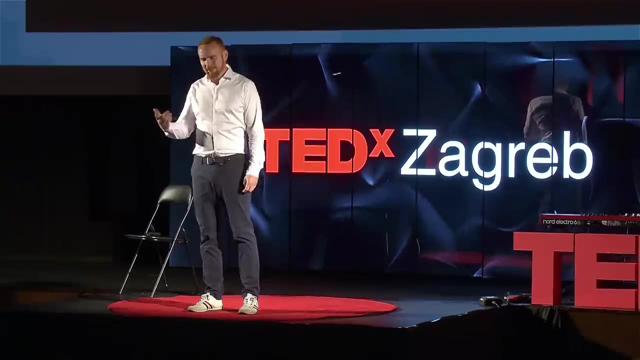 You're happier, You're more content with life And you actually are more relaxed in situations like this. So I asked myself: am I a Duquesne smile? Am I a Duquesne smiling person? And to figure that out, I walked over to my computer. 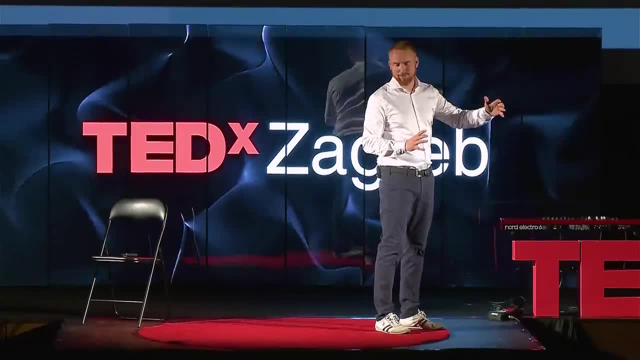 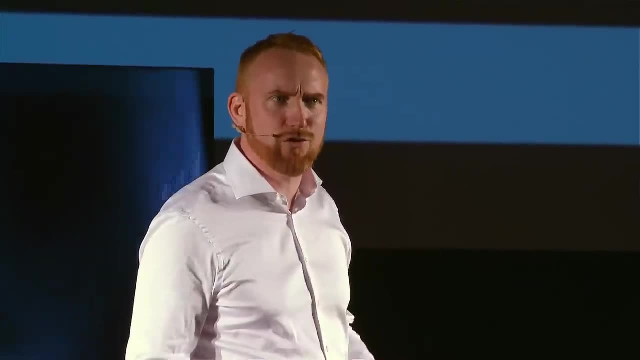 and I logged in and I looked at all my 60,000 Google photos. They're not all of me, but of family members and others. I looked at mine and it seemed like my brain required, short of a miracle, to do a Duquesne smile. 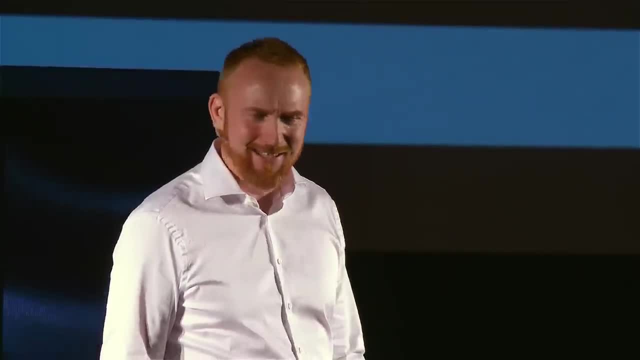 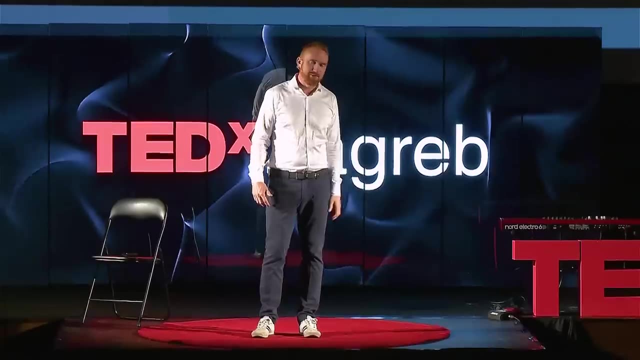 You know where you smile with your entire face. I thought that's not fair And, considering the psychological benefits, I better learn this. So I spent not four but six months learning how to do a Duquesne smile And suddenly my brain was launching. 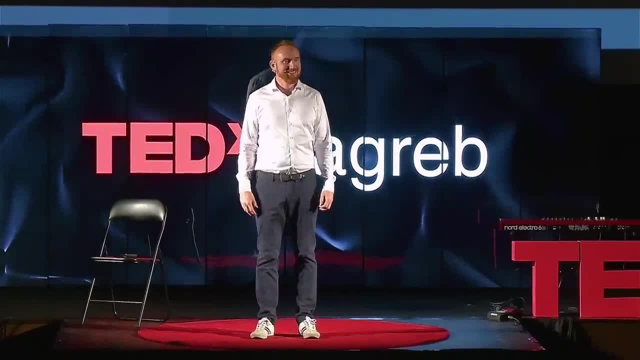 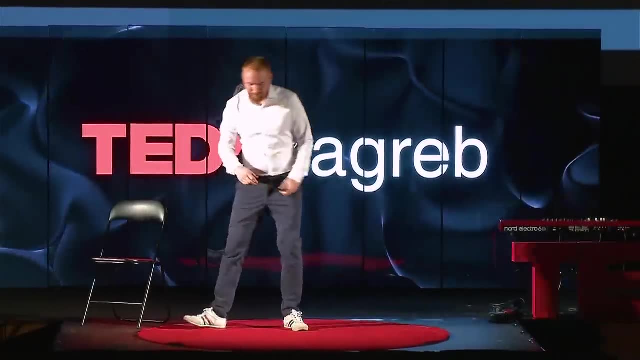 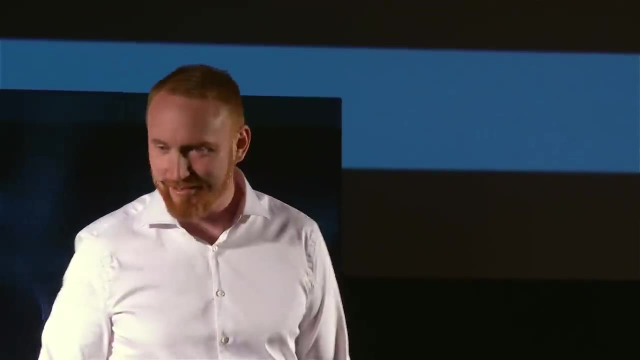 Duquesne smiles in just everyday happiness. It's beautiful And I felt happier as a human being. I want to show you what it looks like. Every time I go on my summer holidays, I take a photo of myself, And these were the last years. 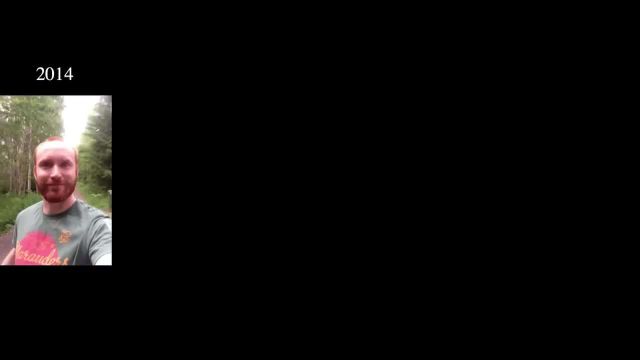 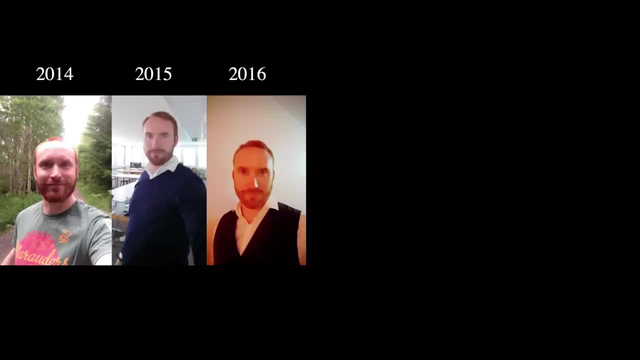 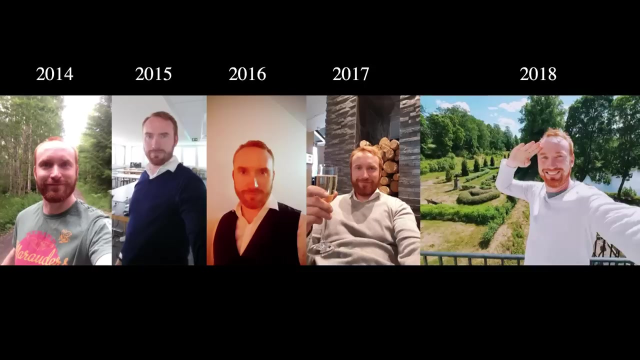 of those photos. This was 2014.. There's no Duquesne smile 2015,. definitely no Duquesne smile 2016,. still no Duquesne smile 2017, no Duquesne smile This year. Duquesne smile. 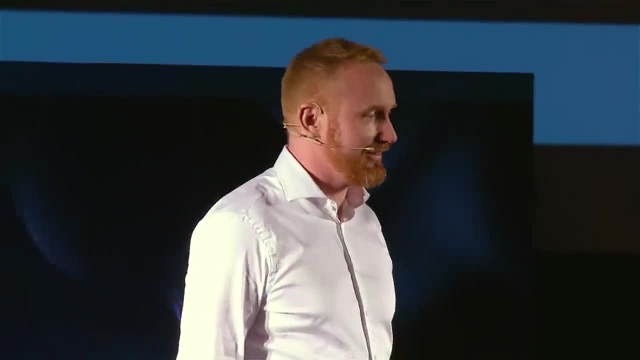 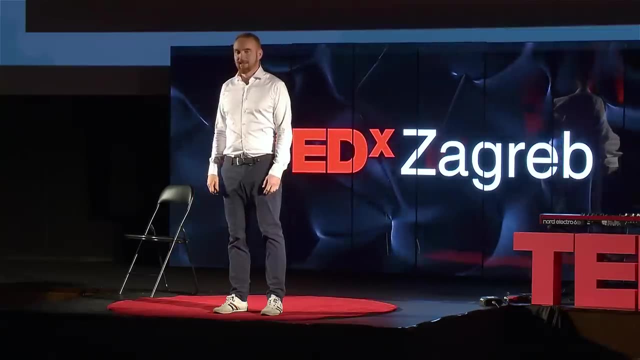 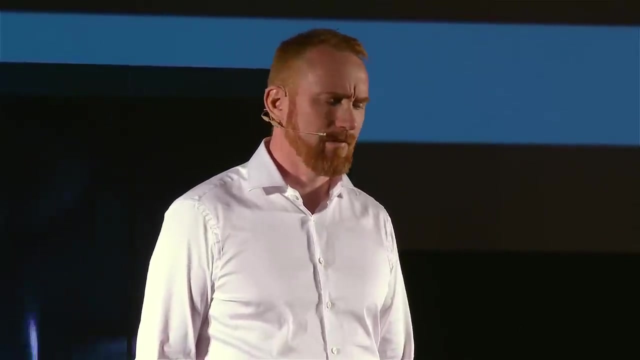 Does it make a difference? Absolutely. It brings joy to you and stability to me. Now we've come to the end of this talk and I would like to end with something that relates to boxing. You know Muhammad Ali and the likes. 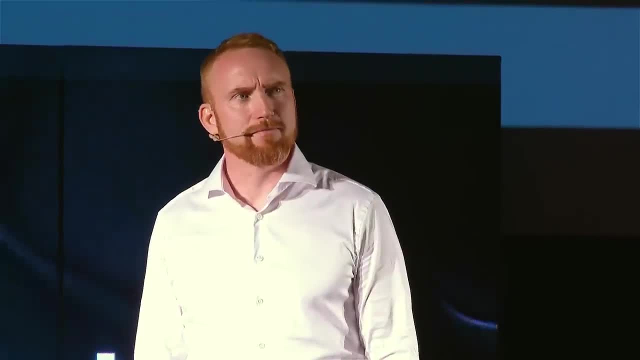 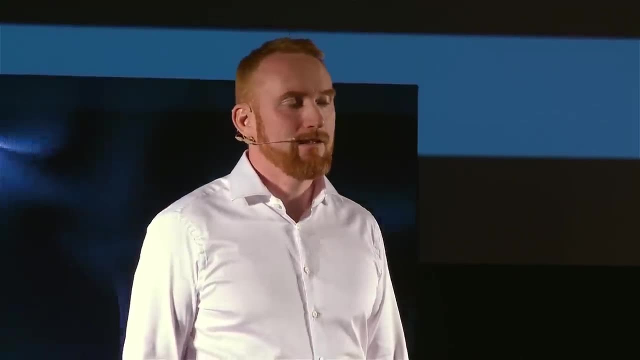 they have combinations for when they're going to strike somebody, knock out, And the same kind of combinations exist in public speaking as well. So what I'd like to show you is this combination. I'm going to start with the number 34,. 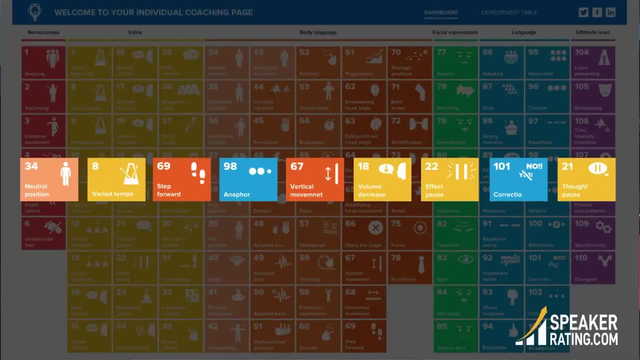 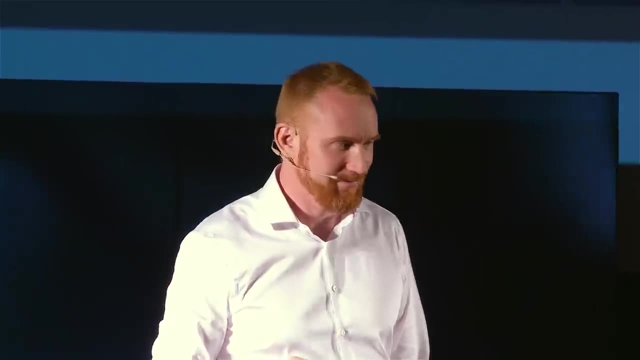 go to number 8,, and then we'll carry on to 69, and 98, and 67, and 18,, 22, and 101, and 21.. Are you ready for the combination? Okay, looks like this. 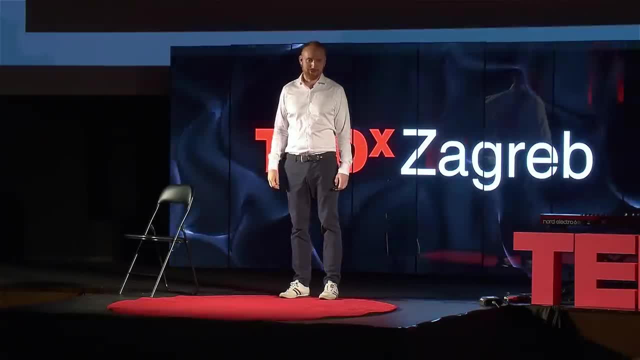 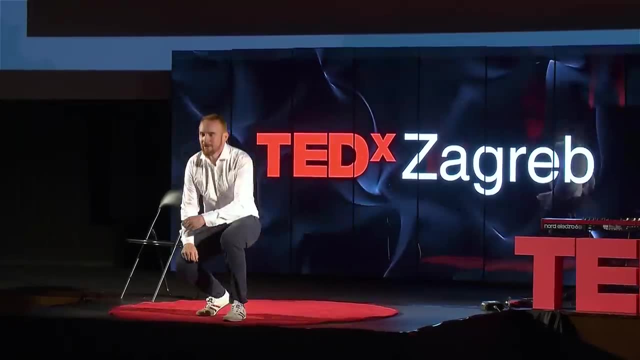 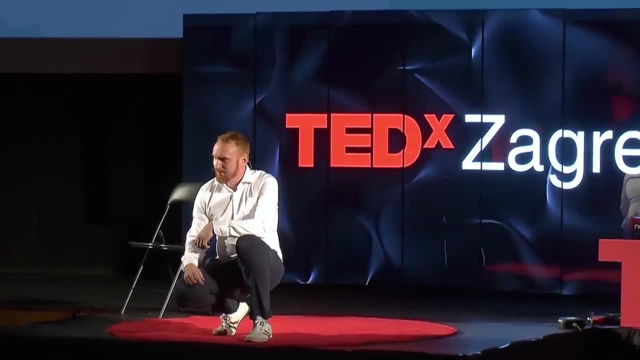 Ladies and gentlemen, I hope that you've had fun, that you have learned, but more than anything, I hope that you feel inspired to become a greater public speaker, because anybody can become good, anybody can become great and everybody can become outstanding. 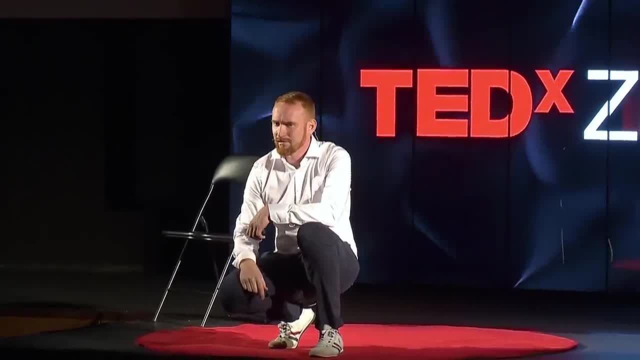 because it all comes down to one single thing. Thank you.